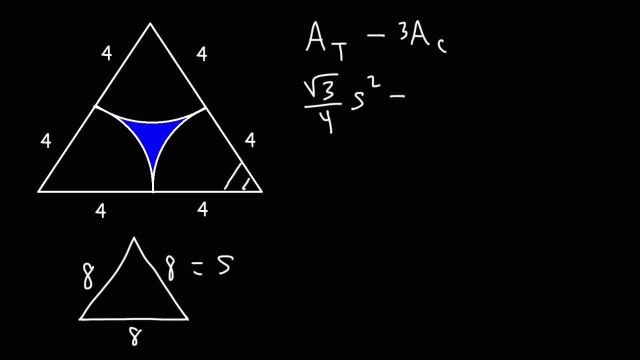 Now how can we calculate the area of this portion of the circle? So this is known as a sector of a circle. To calculate the area of a sector of a circle, we could use this formula: The area of an entire circle is pi- r squared. 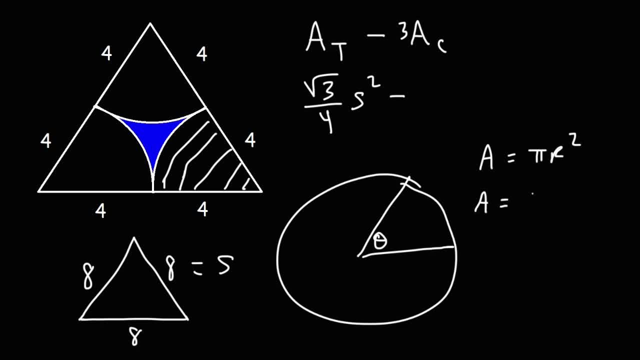 So the area of just a sector of the circle is going to be theta divided by 360 times pi r squared, where theta over 360 represents a fractional part of the entire circle. So this is the area of a sector of a circle and we could use this formula to calculate the area. 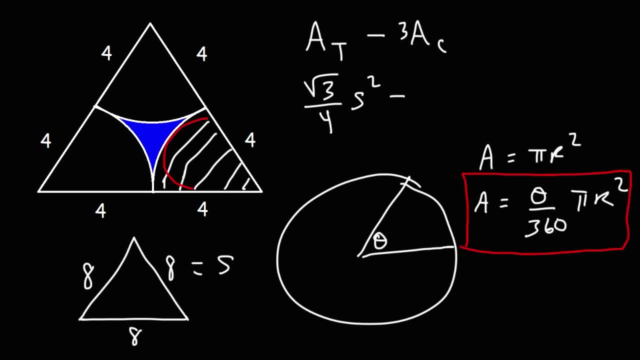 highlighted in red will give us the area of just one sector of a circle. Well, we have three sectors, so we're going to multiply it by three, So this would be a sub c: the area of just one sector of a circle. So it's going to be 3. 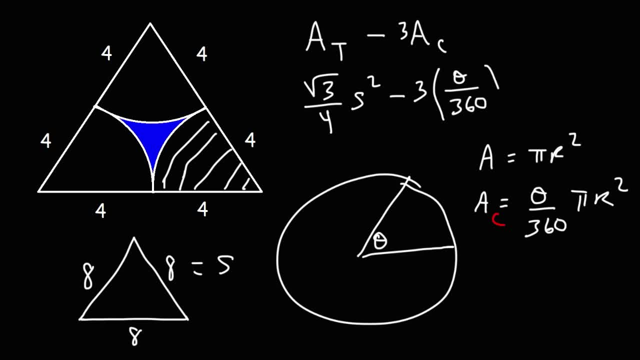 times theta, over 360 times pi r squared. So at this point we have everything that we need to get the answer. So we just need to do the work. So we have the square root of 3 over 4 times s squared. 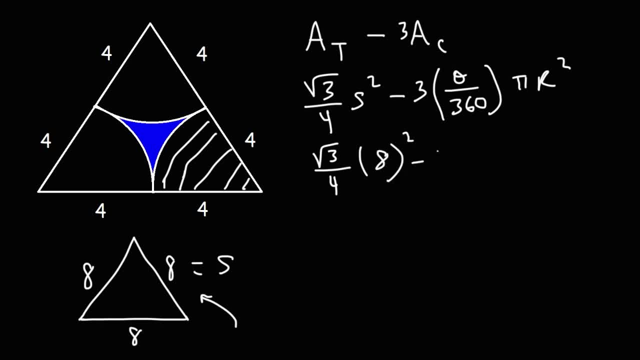 s is 8.. So this is going to be 8 squared minus 3.. Now what we need to find is the angle. What is the angle of this sector? What is the angle of an equilateral triangle? Now, the three angles of a triangle must always add to 180.. 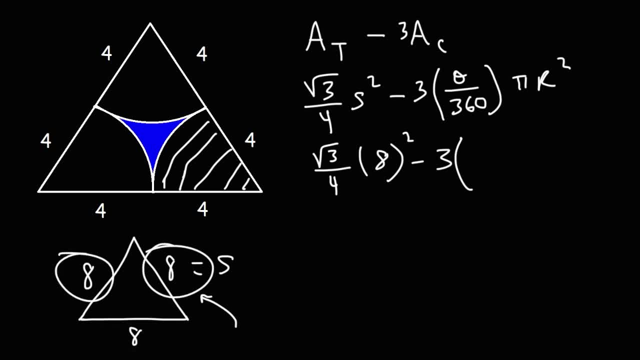 Because all three sides are the same, the three angles are equal to each other. So because they have the same measure, we can call it x, x plus x plus x must equal 180. So that's 3x is equal to 180.. Dividing both sides by 3, we got x is equal to 180 over 3,. 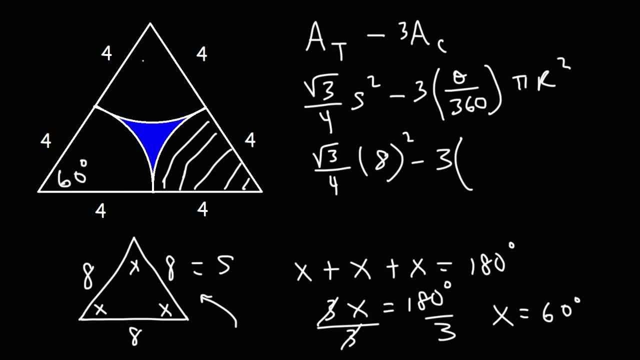 which is 60 degrees. So the angle for each sector is 60.. So we're going to replace theta with 60 divided by 360 degrees And then multiplied by pi times the square of the radius. So the radius of each circle that's inside of the triangle is 4.. 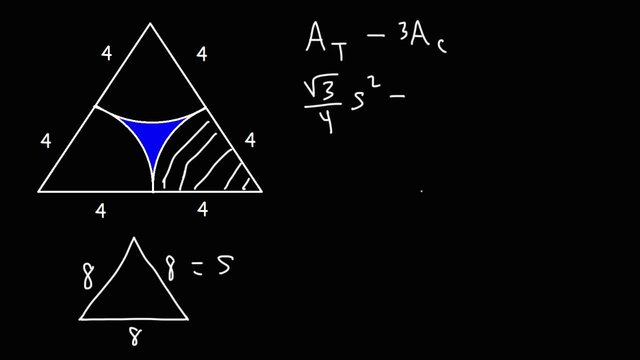 a sector of a circle. To calculate the area of a sector of a circle, we could use this formula: The area of an entire circle is pi r squared, So the area of just a sector of the circle is going to be theta divided by 360 times pi r. 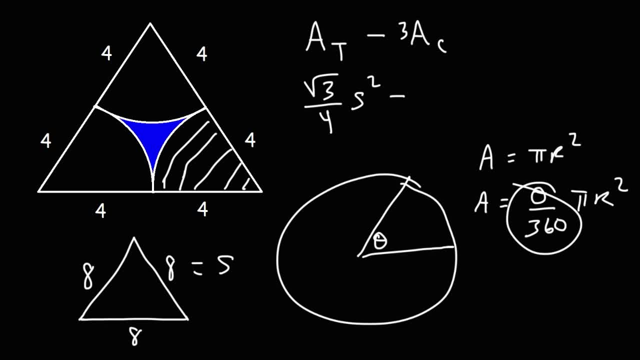 squared, where theta over 360 represents a fractional part of the entire circle. So this is the area of a section of a circle. We could use this formula to calculate the area of. this formula highlighted in red will give us the area of just one sector of a circle. 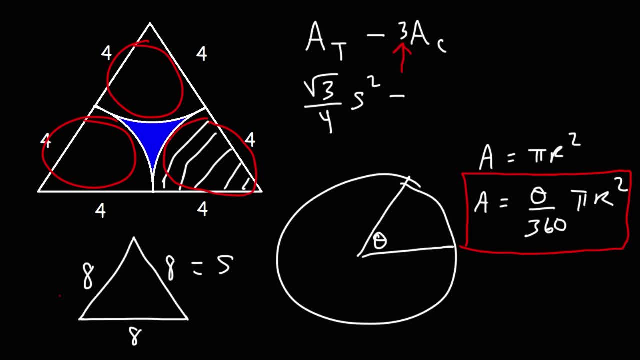 Well, we have three sectors, so we're going to multiply it by three, So this would be a sub c, the area of just one sector of a circle. So it's going to be three times theta, over 360 times pi r squared. So at this point we have everything that we need. 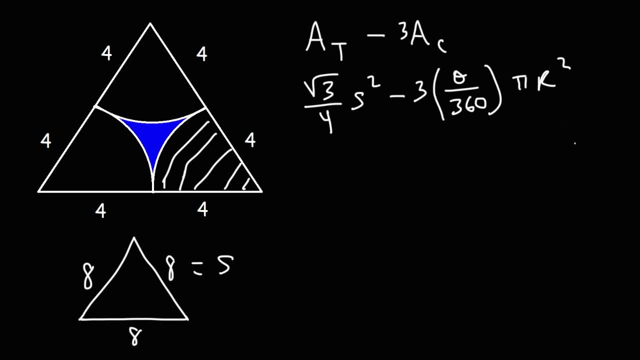 to get the answer. So we just need to do the work. So we have the square root of three over four times s squared s is eight. so this is going to be eight squared minus three. Now what we need to find is the angle. What is the angle of this sector? 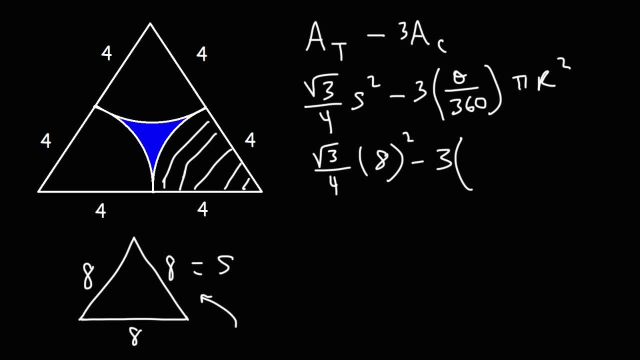 What is the angle of an equilateral triangle? Now, the three angles of a triangle must always add two: 180.. Because all three sides are the same, the three angles are equal to each other. So because they have the same measure, we can call it x, x plus x plus x must equal 180.. 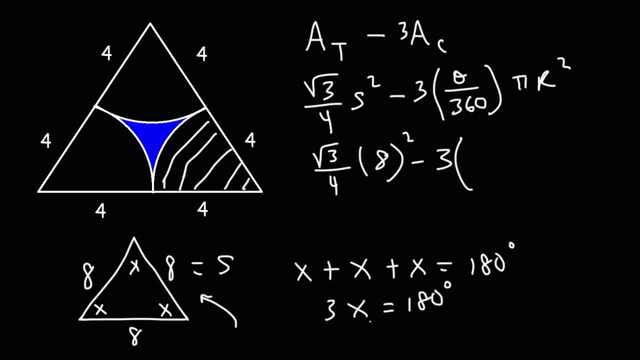 So that's three. x is equal to 180.. Dividing both sides by three, we got x is equal to 180 over three, which is 60 degrees. So the angle for each sector is 60. So we're going to replace theta with 60, divided by 360 degrees. 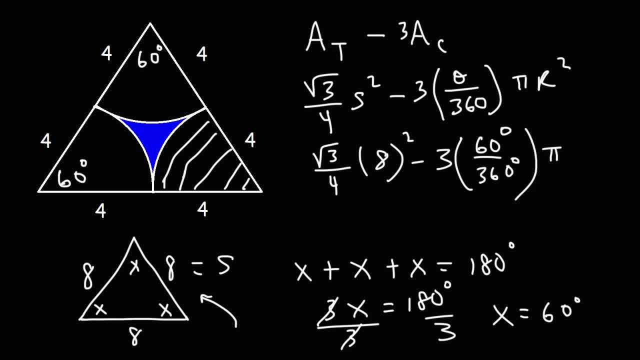 and then multiply it by pi times the square of the radius. So the radius of each circle that's inside of the triangle is four. So this is going to be pi times four squared. So the area of the shaded region is going to be the square root of three over four. 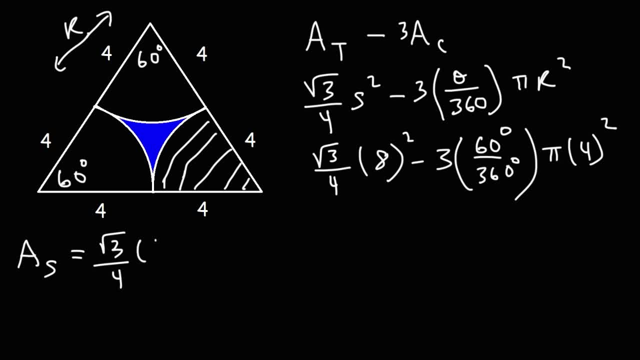 So we get pi times eight squared. Eight times eight is 64.. And then three times 60 is 180.. And then we have pi times four squared. Four times four is sixteen. Now 64 divided by four, that's sixteen. 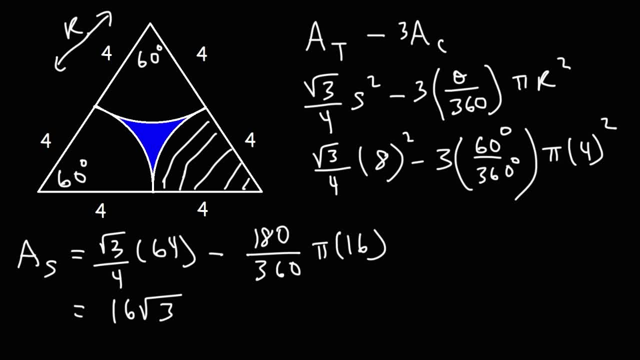 So this is 16 square root three, 180 divided by 360, we can cancel a zero, so it becomes 18 over 36.. Now, 18 over 36, we can reduce that 36 is 18 times 2, and 18 is. 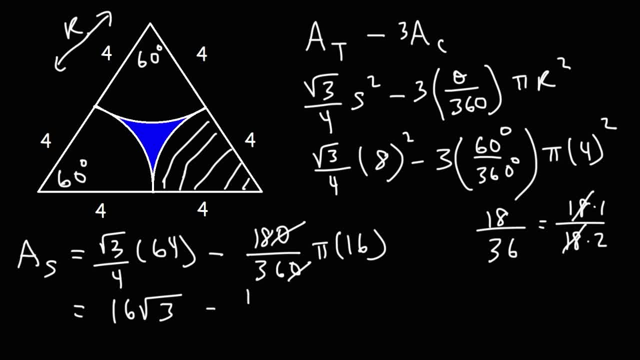 18 times 1, so it becomes 1 half. So we have 1 half pi times 16, and half of 16 is 8.. So we can write the final answer as 16 times the square root of 3 minus 8 pi. 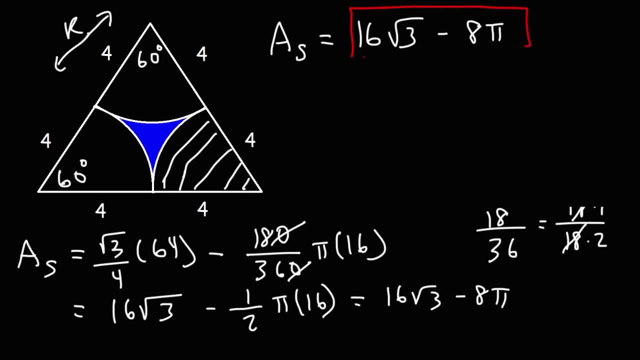 So this is the exact answer. That is the area of the shaded region. Now, if you want to get the decimal value of that, I'm going to give it to you in just a second. So let me type this in: So this is equal to 2.58 square units. So that is the area of the shaded region. 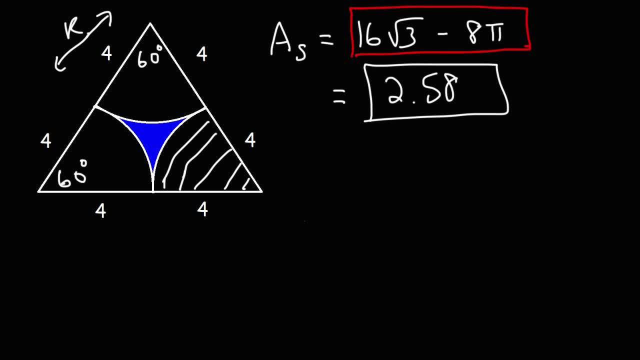 So that's it for this video. So now you know how to solve this particular problem. Thanks for watching. 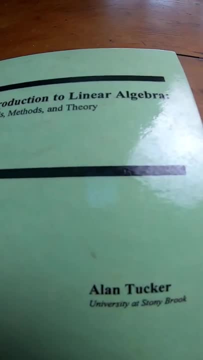 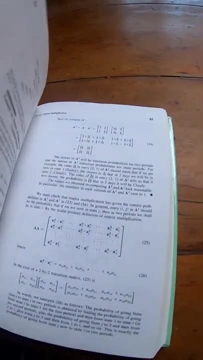 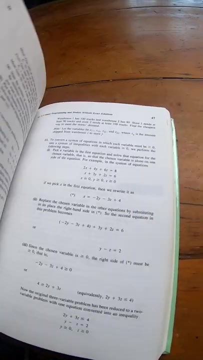 Introduction to Linear Algebra Models, Methods and Theory by Alan Tucker University at Stony Brook. So this is a pretty good book on linear algebra. I have read parts of it. I feel like, even though it's supposed to be an introductory book, when I was reading it I did have a hard time. 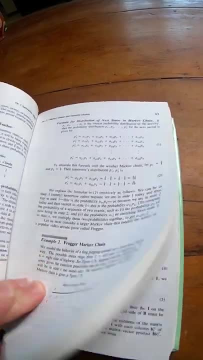 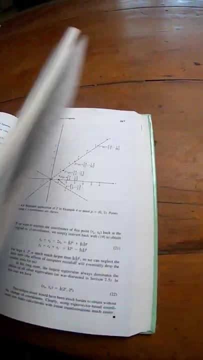 I haven't looked at this book recently, I'll be honest. I just remember when I was learning linear algebra, I tried to use this book and I struggled. I don't think it's a bad book, I just think it's an okay book.